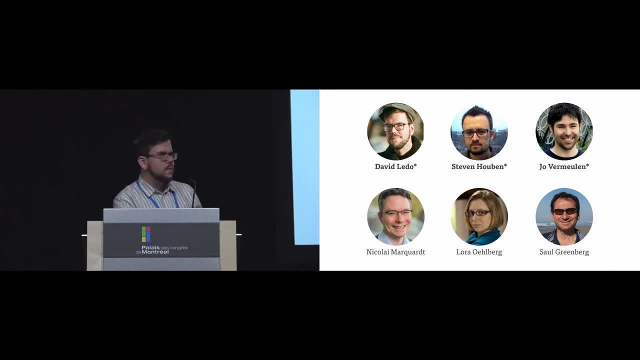 Nicolae Marquardt, Laura Olberg and Saul Greenberg, And you'll notice there's a bold and stars on our names on top, and that's because Stephen Jo and I contribute equally to the work. So the message of this talk is that, despite 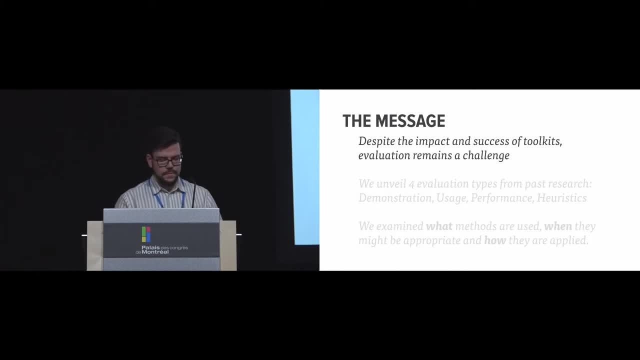 the impact and success of toolkits. evaluation remains a challenge. We unveil four evaluation types based on past research: demonstration, usage, performance and heuristics, and we examine what methods are used, when they might be appropriate and how they are applied. 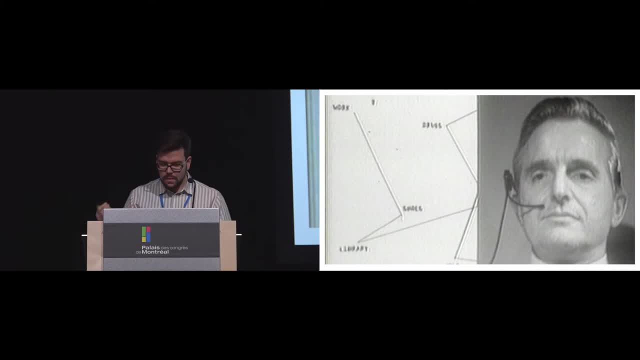 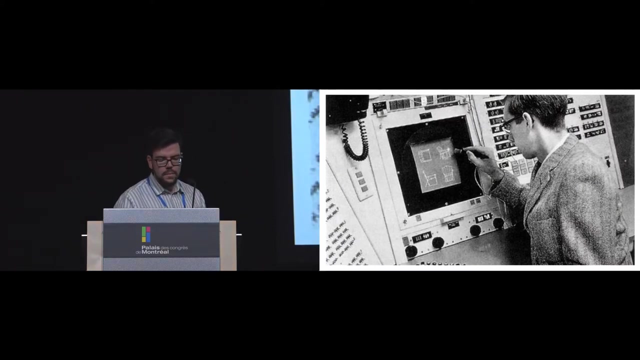 So, as you all know, the mother of all demos is turning 50 years old now, and it's really interesting because it paved the way into how demonstrations can be used as a way to communicate a technology's concepts and ideas, And this kept going all the way through other 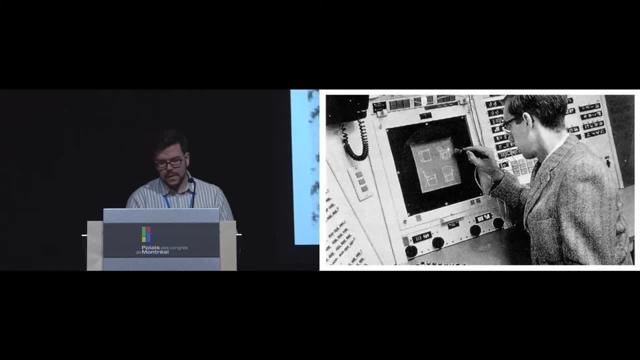 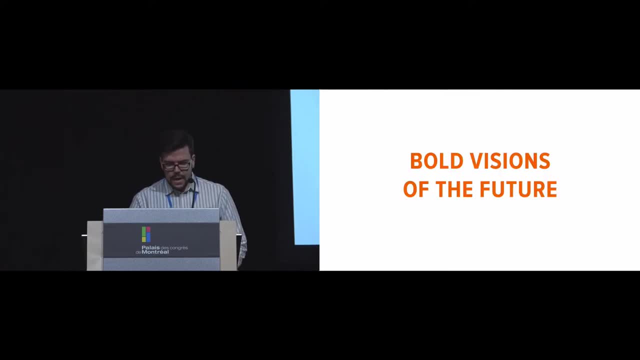 projects like Sketchpad by Sutherland, as well as Ubiquitous Computing Projects at Xerox Spark, led by Mark Weiser. And what's interesting here is that by creating toolkits, it is possible for us to actually create these bold visions of the future, So we can actually author them and then see what they'll be like before they. 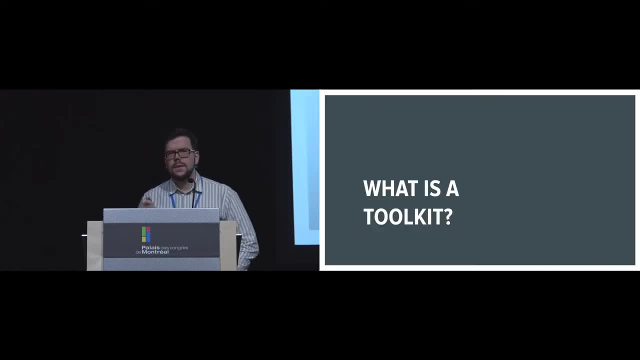 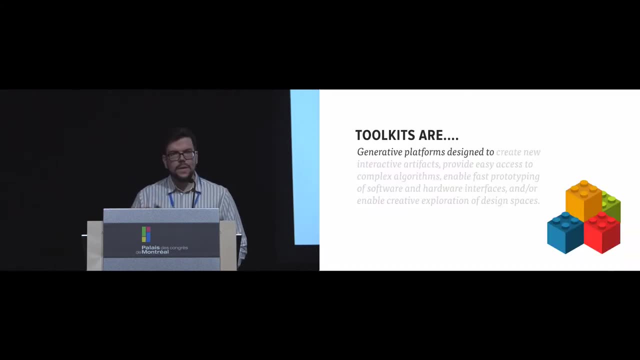 can actually come into play. So I'm using the word toolkit and I thought I would define it first. So what do I mean by toolkit? So toolkits are generative platforms designed to create new interactive experiences and artifacts, provide easy access to complex 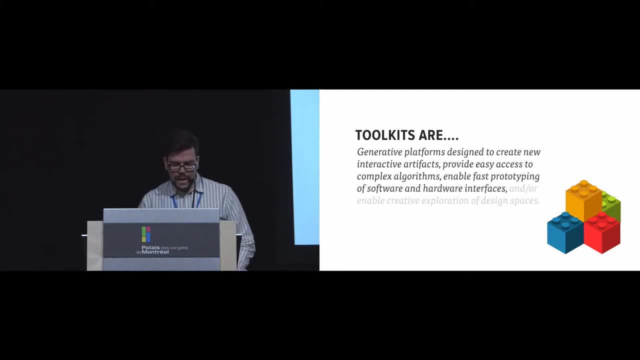 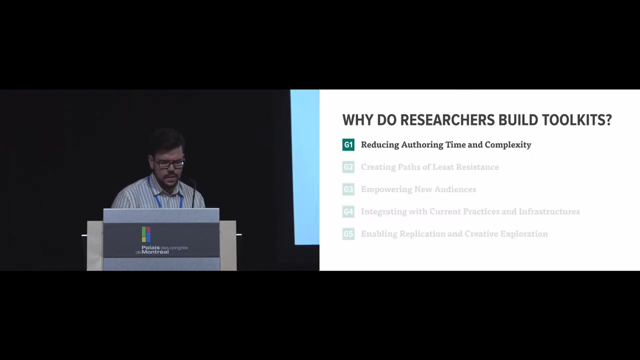 algorithms enable fast prototyping of software and hardware interfaces and or enable creative exploration of design spaces, And they're used in many areas of HCI, such as graphical user interfaces, information visualization, tangible user interfaces and UbiComp. So why do researchers build toolkits in HCI? So the first reason is to reduce authoring. 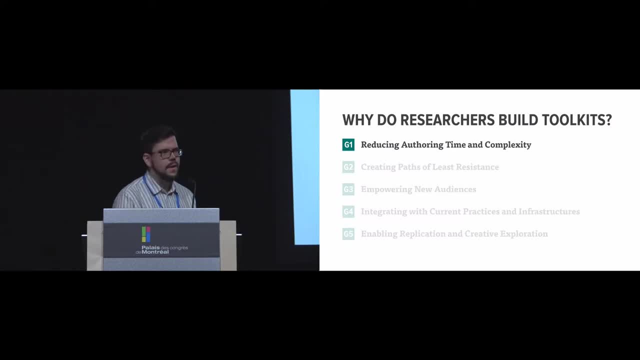 time and complexity. So this idea that we can encapsulate concepts and simplify expertise. Second, it allows us to create passive least resistance, which means that we're able to move people towards the right solutions and away from the wrong ones. It also allows us to empower new audiences. 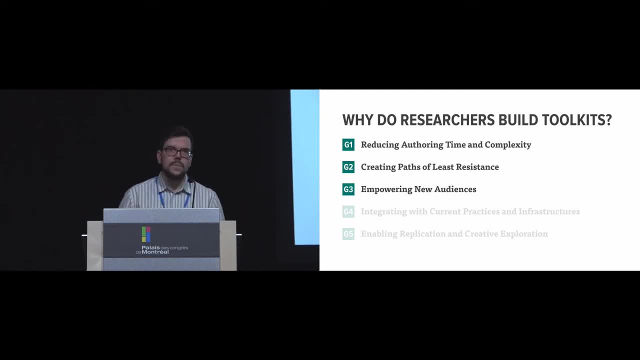 so we can have new participants work in these areas, And one great example of that is how we can move from developers creating user interfaces to designers by having interface builders. It also helps integrate with current practices and infrastructures, so it means that we can align our ideas. 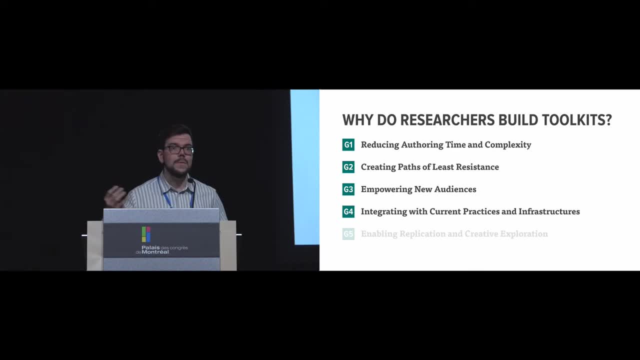 to existing infrastructures and standards, And one example of that is D3 and how it was integrated into the current web standards. And finally, it enables replication and creative exploration, So it allows people to replicate different ideas that can come together into a suite of tools. 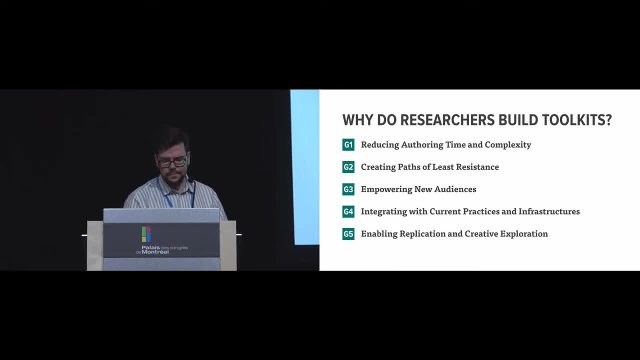 that can explore an area and create more powerful solutions than ever before. So essentially, all of these goals are trying to get to this idea of opening new solution spaces. Now the thing is that toolkits can create many different solutions by using, reusing, 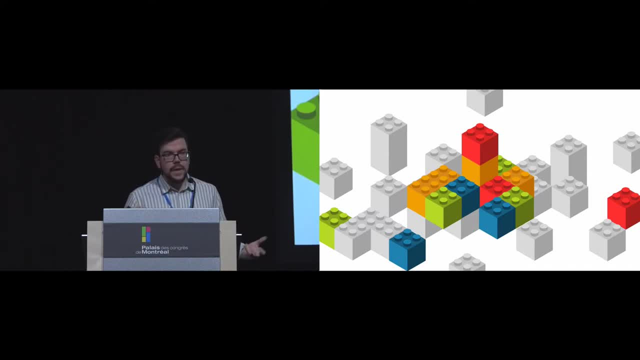 and combining the different solutions from different building blocks, And this leads to a very large space, but the trade-off to that is that, because we have this generated power, there's a large space that remains underexplored, And so the question is how we can go back. 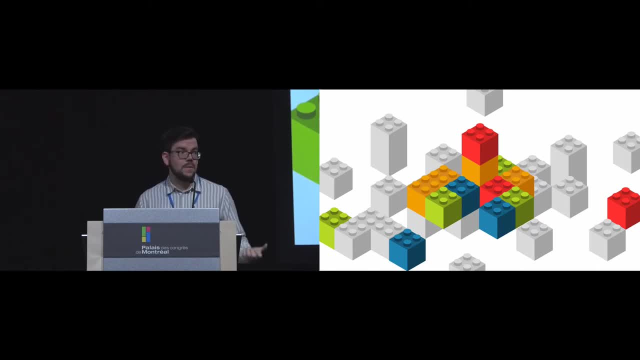 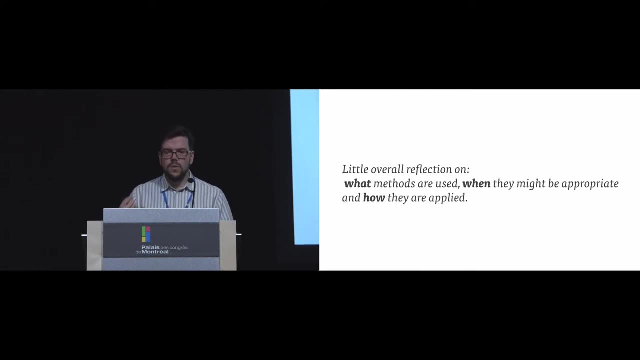 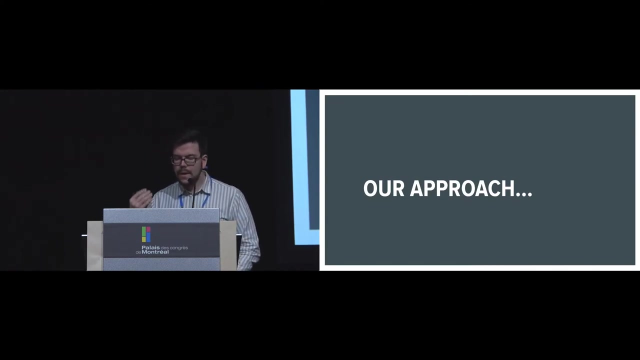 to these original goals that we established and know that we actually met them. So we found that there's very little overall reflection on what methods are being used, when they're appropriate and how they might be applied. So we wanted to get more insight and find a way to have 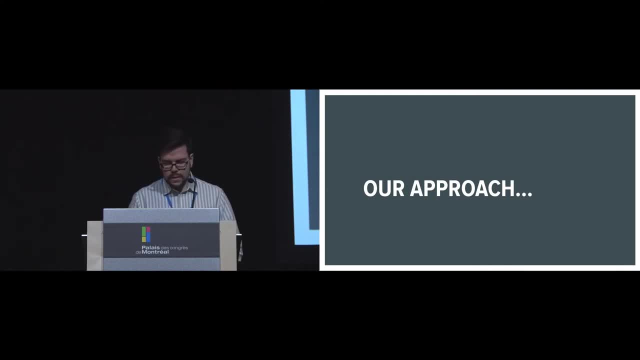 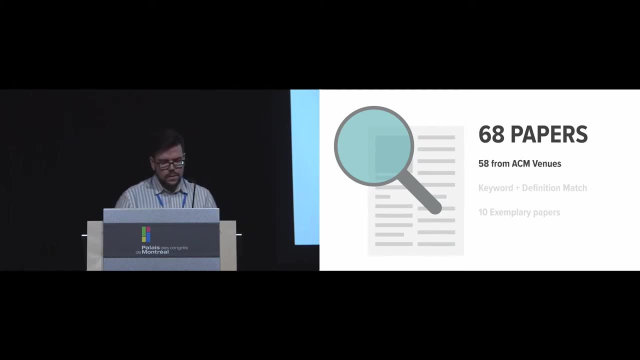 an informed discussion about this so that we can actually understand this. And so what we did was we looked at 68 representative papers- 50 of them were from ACM venues, and we applied a keyword and definition match and we ensured that we also took 10 additional papers. 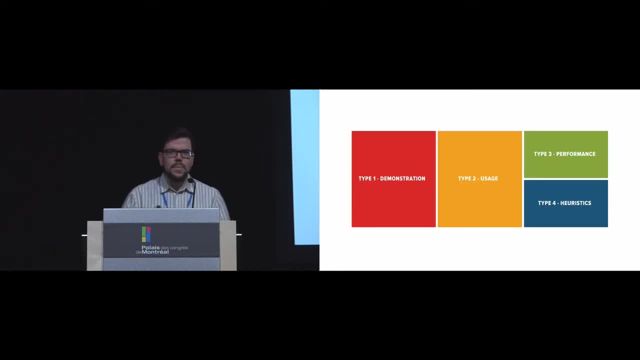 that were also exemplary From that. we applied open coding and focus coding, and then we did thematic clustering and we found four different types of evaluation- Demonstration, usage, performance- and then we applied the results and heuristics. So our data looks something like this: 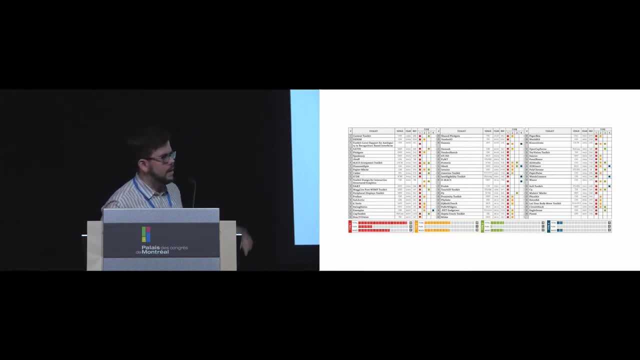 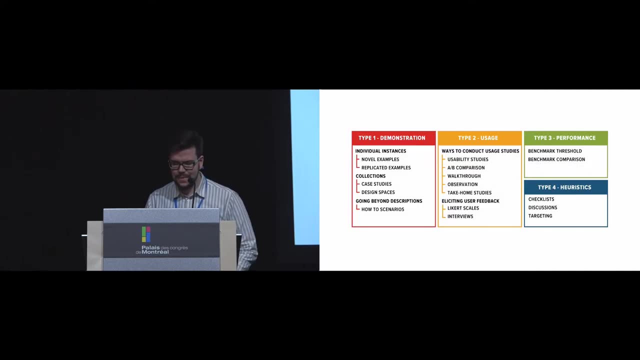 You can find that in our paper. Essentially, you can see all of the different toolkits and how they use different methodologies and how they come together, and some descriptive statistics as well. So I'm going to go over the different types of evaluation. 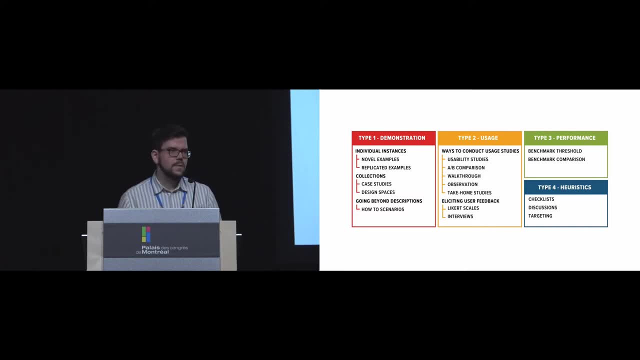 and I will also apply and look at our own observations and reflections. In our paper we actually discuss some of the challenges. I won't go into those because of time restrictions, but hopefully you have a time to look at that later. Thank you. 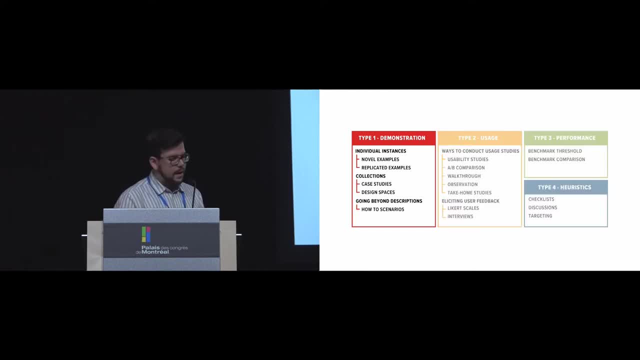 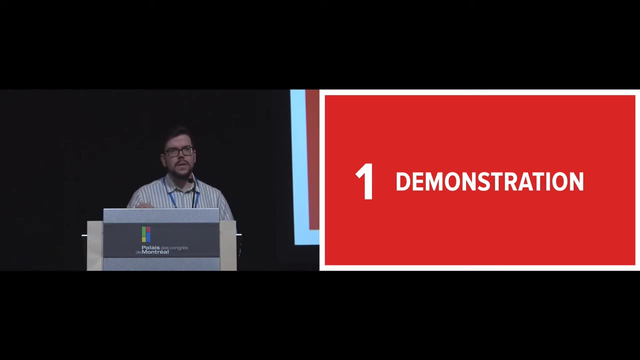 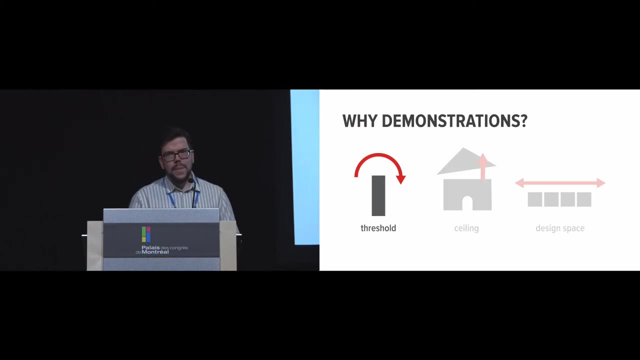 So I'll start by looking at demonstrations, And essentially the idea of demonstrations is that people create examples and scenarios that can clarify how a toolkit's capabilities come together and can enable people to create these claim applications. So by doing that, they can show how these different building 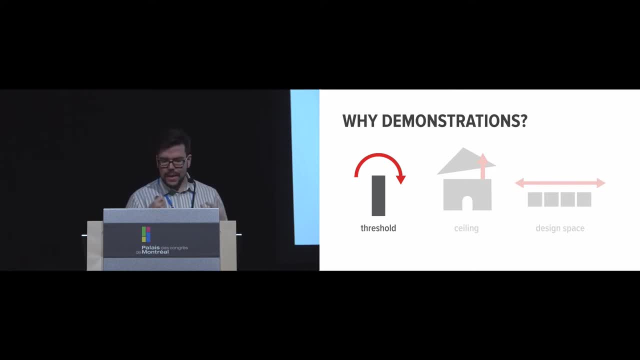 blocks are coming together and creating these paths of least resistance, And they can also show the different workflows and how they're actually demonstrating that solution space that we talked about, And through that they can show things like the threshold or how easy it is to get started. 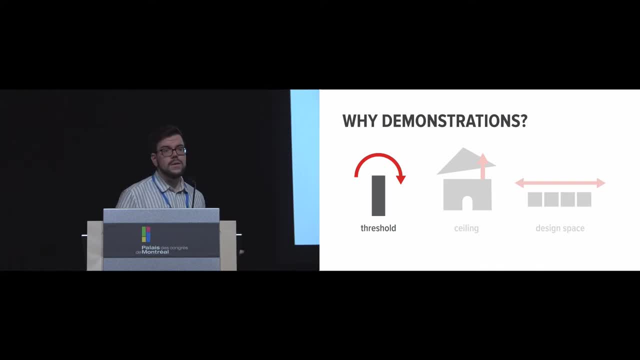 They can show the ceiling or the complexity of the application, Or they can go as far as to show the design space and the different breadth of things that they can do and how they fit a larger research team. One way of doing that is through novel examples. 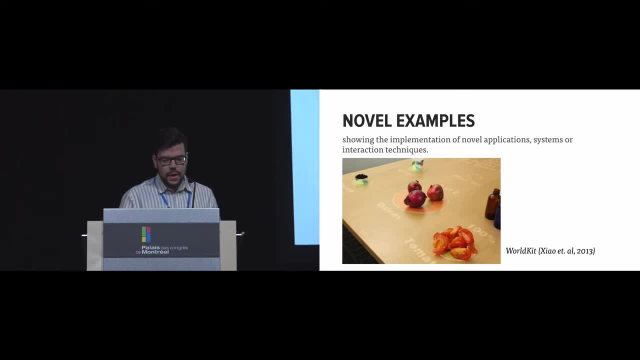 So, for example, they can show implementations of novel applications or interaction techniques, such as it was done in WorldKit, where they actually overlaid projections on top of different objects. Or one might choose to replicate existing examples, So that way they can show that one can author systems. 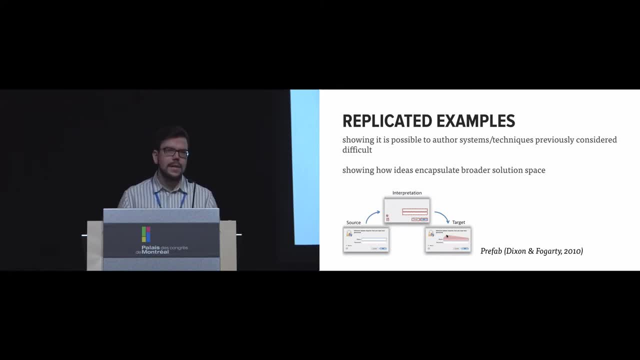 and techniques that were considered difficult and show how these ideas can encapsulate the broader solution space. So one example of that is prefab, And in prefab the authors show how they can integrate very sophisticated interaction techniques that were really difficult to implement into everyday infrastructures just by reverse engineering. 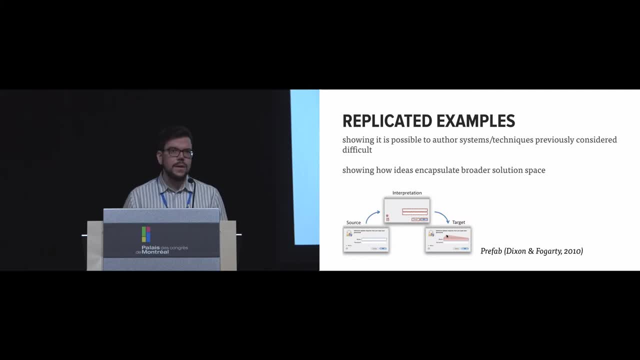 the pixels of the display, And so they can actually integrate all of these without actually having to modify anything. And it's really interesting Because a lot of authors have already started these types of discussions. So, for example, in Perfuse- hearing colleagues actually- 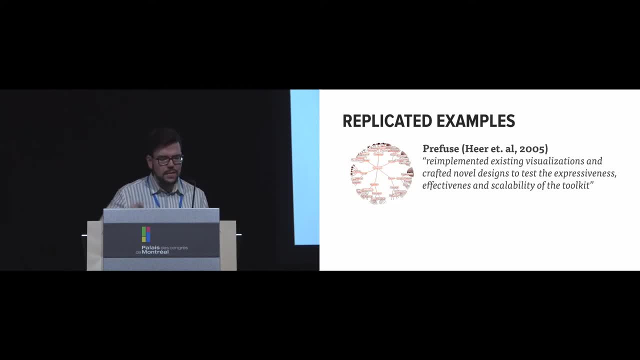 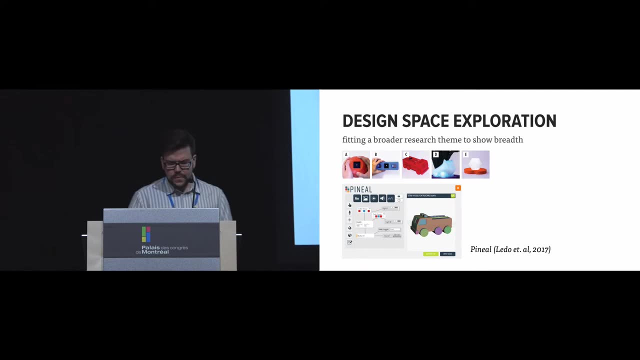 say that they re-implemented existing visualizations and crafted novel designs to test the expressiveness and the effectiveness, as well as the scalability of their toolkit. One might also explore the design space. So it's this idea of fitting the ideas into a broader research. 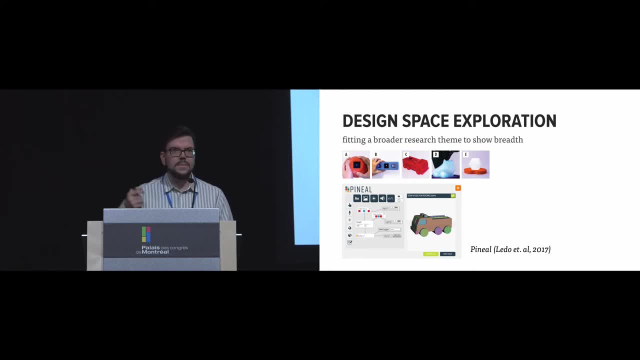 theme. So in Pinio, for example, there's a design space exploration of how to author passive objects that can become smart by adding a mobile device and looking at how sensors are integrated or repurposed. One might also do how-to scenarios. 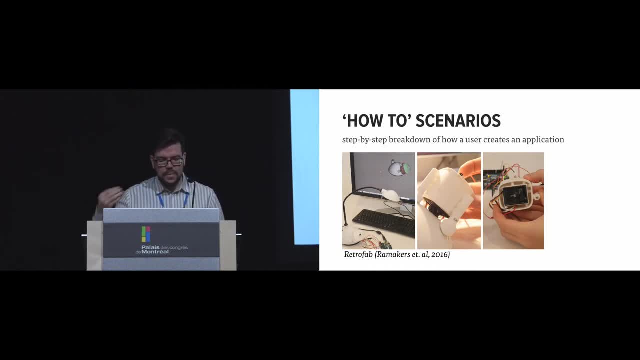 so having this step-by-step breakdown of how to use the application, And so retrofab here has examples of how to retrofit appliances and make them into IoT-compatible objects, So they actually describe how the application would use it, as if you had an end user working with it. 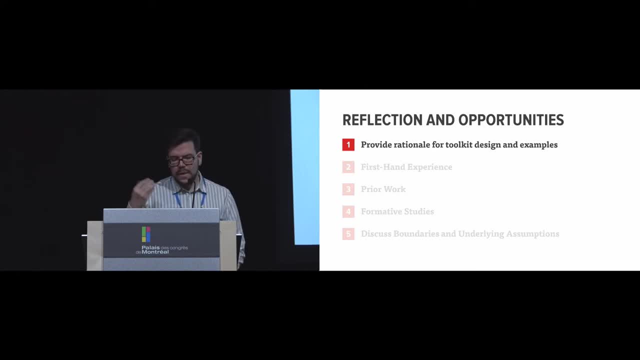 So in our own reflections we find a couple of things. One is to provide rationale for toolkit design and examples. So there's a lot of principles that are being used and it's important to clarify where these decisions are coming from, So authors may have their own experience in hand. 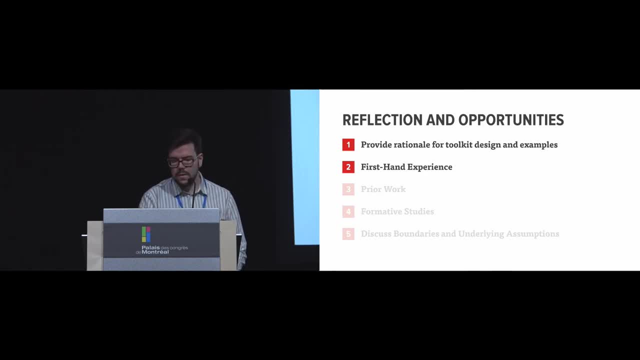 whenever they're creating these tools, so they'll actually understand where the problems are And this inspires or leads to some form of autobiographical design that defines how they're actually creating these solutions. So one example of that is how D3 actually came from the creation. 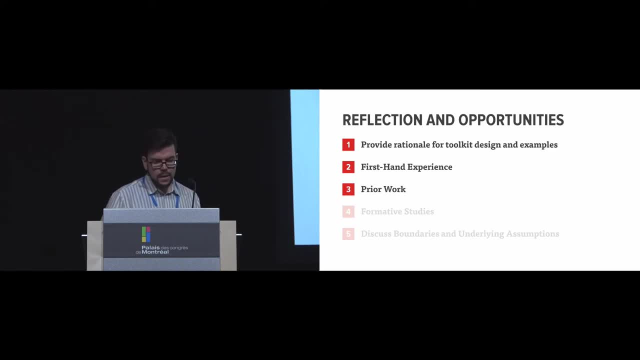 of multiple toolkits in the past. One could also look at prior work and how the research community has determined different problems that need to be solved right now. Similarly, one could also try to understand the intended target audience by using formative studies, And through that they can actually 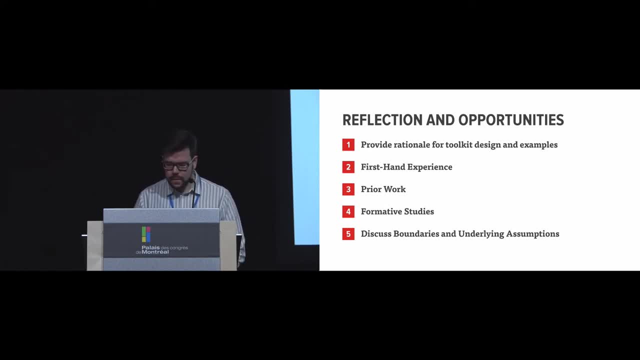 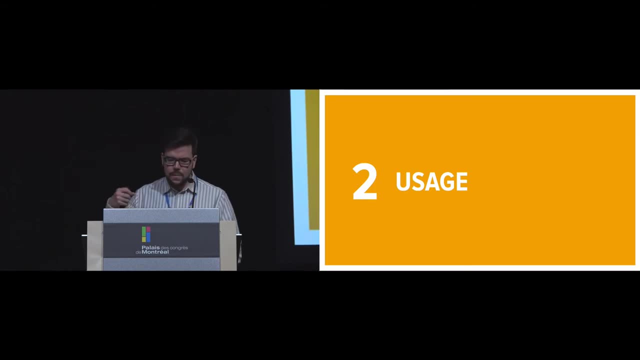 discuss the boundaries and underlying assumptions so that they can explain what doesn't work well and what is actually complicated with the toolkit. So I'll move quickly into usage, which is this idea that one can see who can use the toolkit, as opposed to what the toolkit can do. 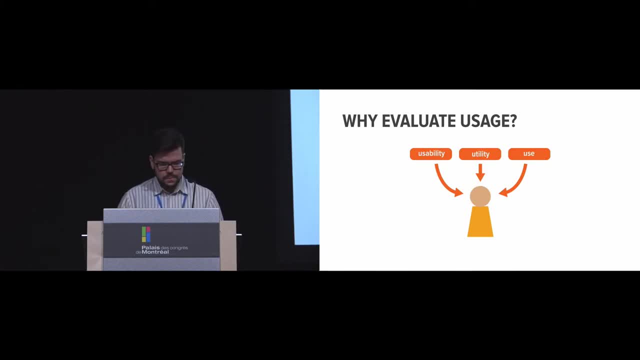 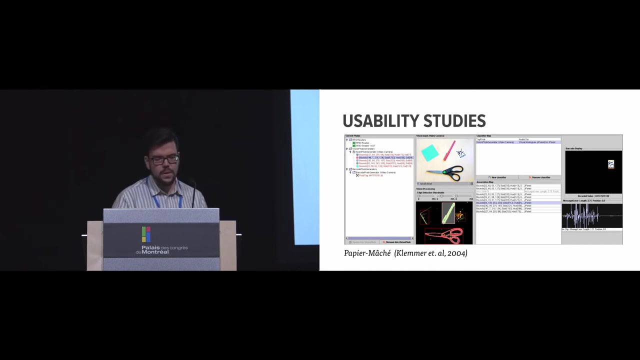 And we can do that through usability, utility and use. So one example here is usability studies, which can look at speed, errors, performance and documentation. So PaperMache actually does an API usability study that finds issues with the documentation, which 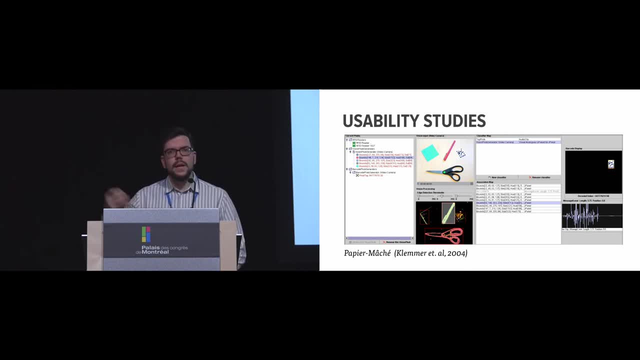 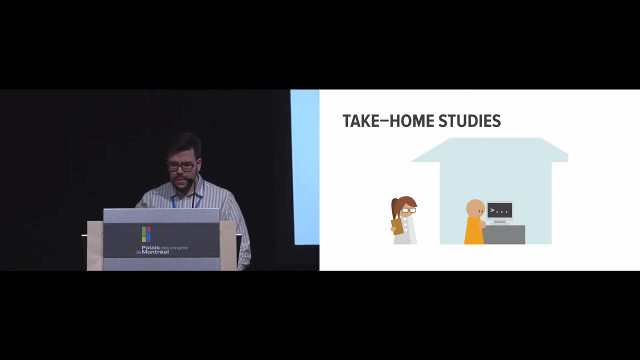 leads to iteration on the actual document and the toolkit itself, PAPERMACHE. People can also take some of these things home to get some external validity. So essentially the idea is that they can do some work on their own, So it's typically given to students, for example. 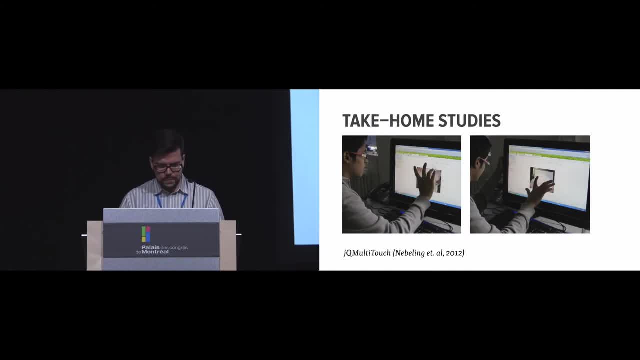 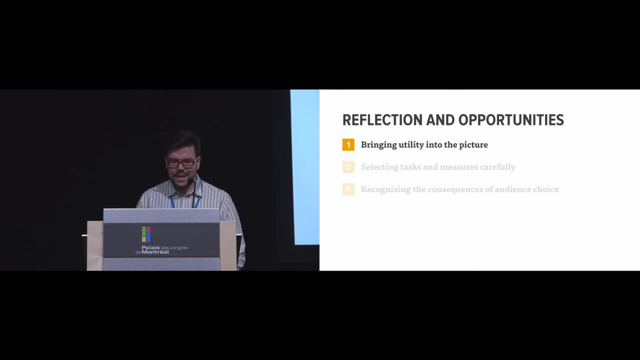 since they'll be early adopters of the toolkit itself. So in that, we can find that one thing that we reflected on was this idea of bringing utility into the picture, because even though a toolkit may be usable, may not be useful. We can select tasks more carefully. 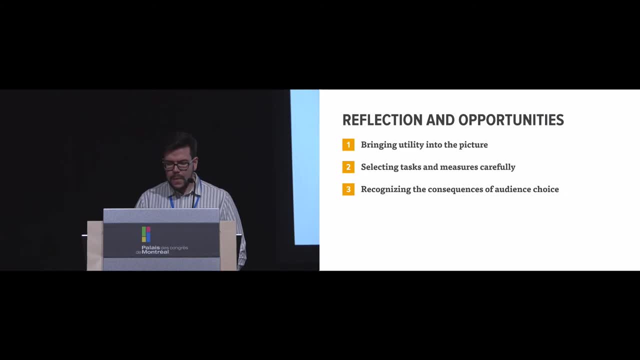 so that they're representative and the measures can be appropriate to the claims made in the paper And we can recognize that the consequences of the audience choice matter. So things like having undergrads do the toolkit may make sense if they're computer scientists. 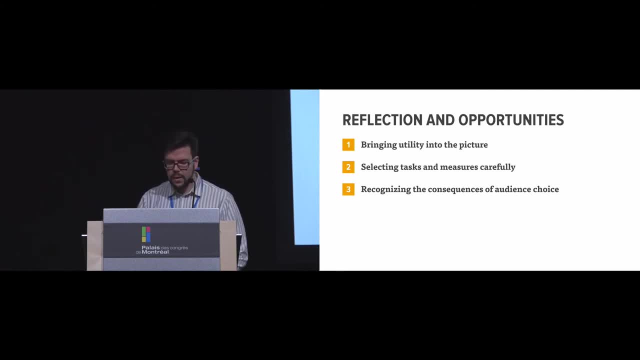 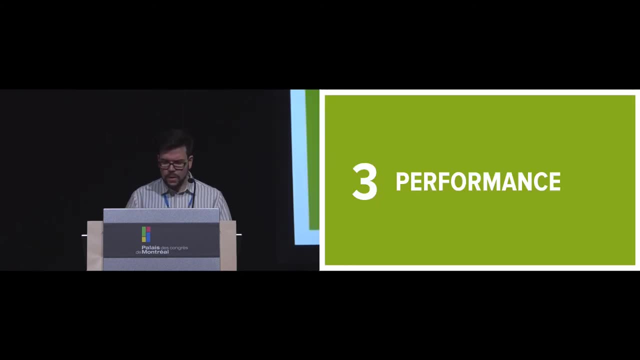 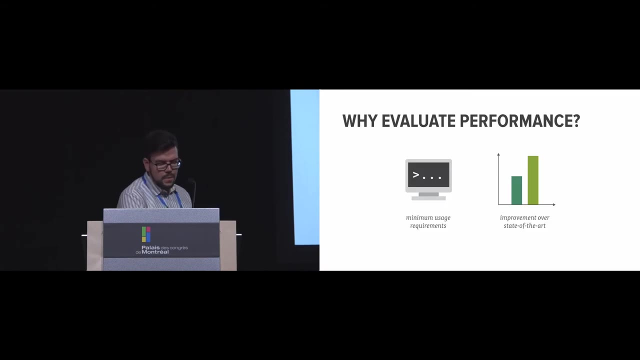 and we can extrapolate that idea to developers. but it may not be the case for other types of evaluation. In terms of performance, instead of looking at what and who, it's about finding how well it works and finding the technical performance. So one can look at the minimum usage requirements. 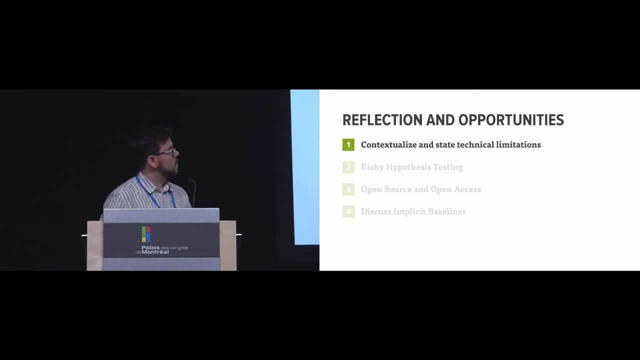 or how things are improved over the state of the art. So some of the reflections include how different goals go from commercial to research toolkits and why these limitations are being used or not. what matters essentially. From there we can do risky hypothesis testing. 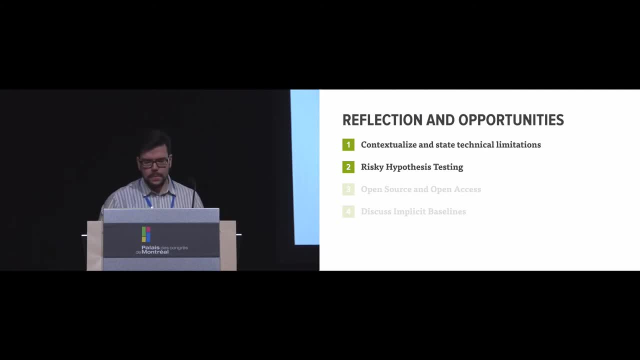 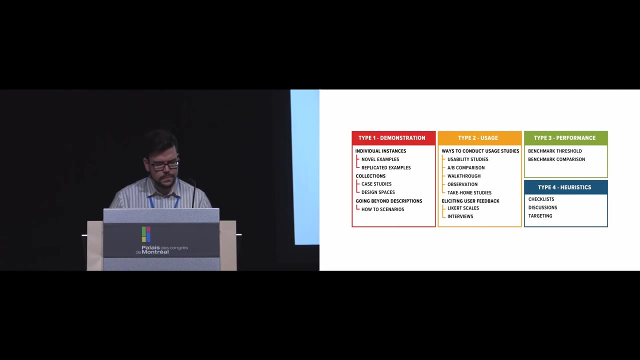 and actually try to see when the toolkit breaks to truly understand the technical boundaries. We can facilitate representation and comparison through open access and we can discuss the implicit baselines, For example, 30 frames per second for camera-based projects. Last thing, I'm gonna talk about heuristics. 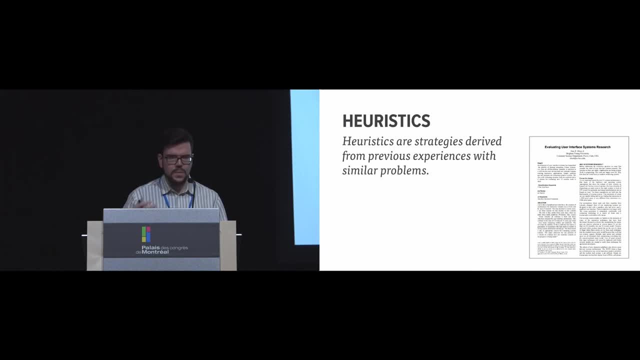 and it's this idea that we have strategies that are derived from previous experiences with similar problems. So a lot of this work often goes to Conrad Dimensions of Notation or Dan Olson's work in evaluating toolkits, And these are based on tried success. 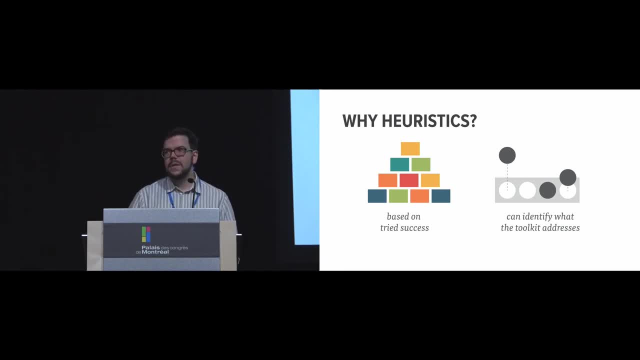 and can identify what the toolkit addresses and what are the limitations. So, for example, one can use these ideas as design guidelines to inform their design early on. They can also use it to inform different evaluation types, so they can actually take these heuristics. 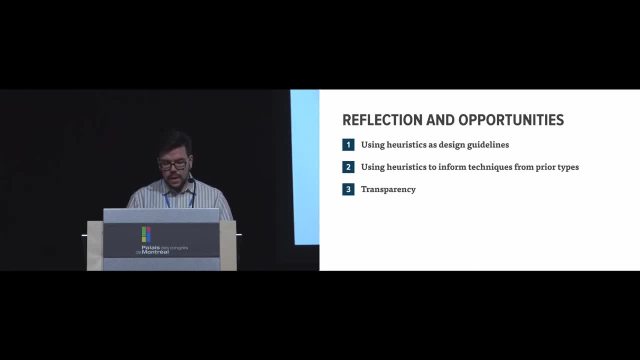 and apply them to define tasks for user studies, for example, And we should be able to be more transparent and distinguish when we're cherry picking versus when we're ignoring relevant heuristics by articulating why we're not including them. So I'm gonna step back a bit. 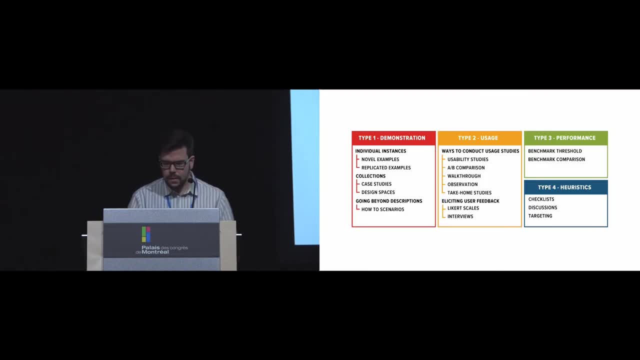 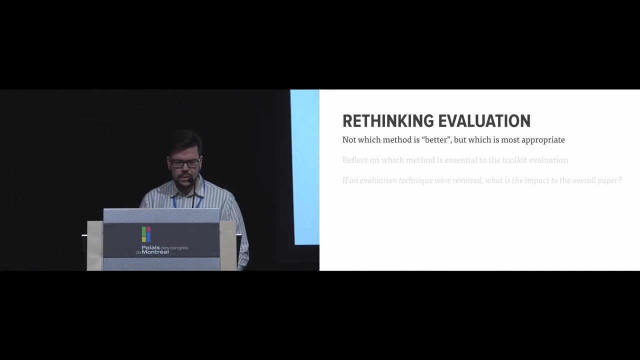 I talked about the four types of evaluation and essentially we talked about these different techniques that are associated, And the first point is this idea of rethinking and evaluation, Because it's not necessarily about which method is better, but which one's the most appropriate. 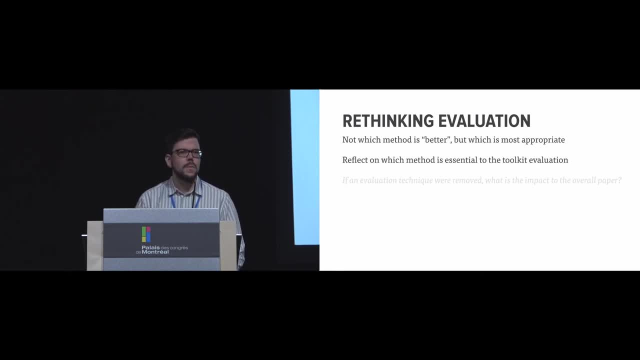 And we had to reflect on which method is essential to toolkit evaluation, And one way of doing that is thinking about what, if we removed that method itself, Will this affect the paper and to what extent will it do that? One point that we had 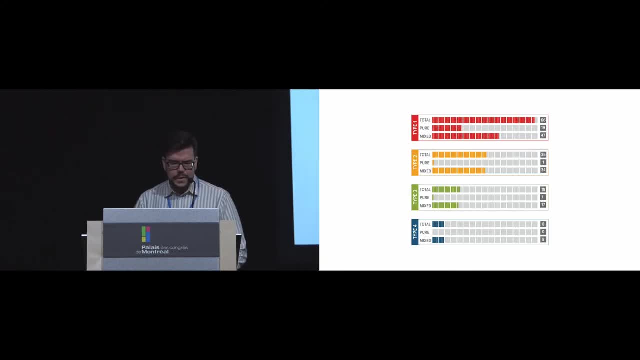 this evaluation by demonstration. If you look at our data, you can see that a demonstration was using almost all of the toolkits, while usability- or sorry, usage as well as performance, were used about half or a third, And demonstration was used on its own. 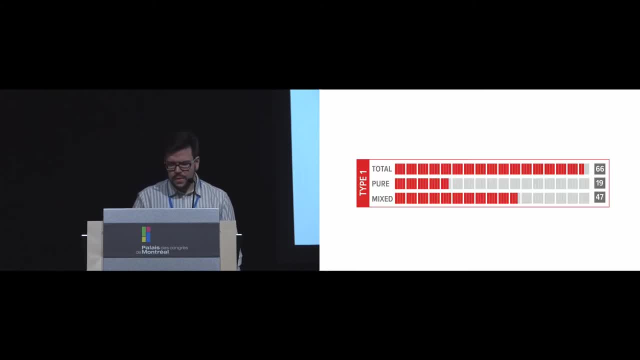 whereas the other ones tended to complement these demonstrations, And so the reason for this is because demonstrations can be an effective way of communicating the toolkit principles and concepts, So it's kind of like your best bang for your buck, in a way. 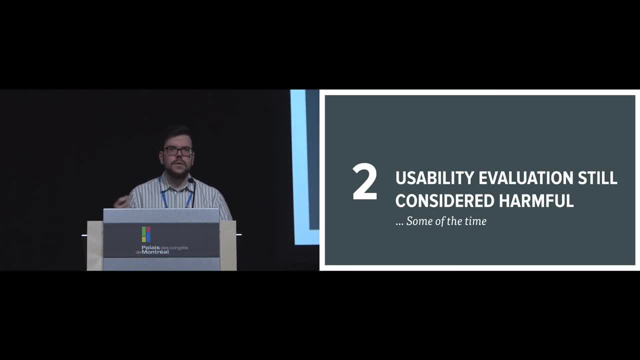 We still found, although there were a lot of really good usability studies looking at creative exploration and so on, there were a lot of papers that are still just tacking usability studies at the end, which have small sample size or nonrepresented groups that don't really show the passive least resistance. 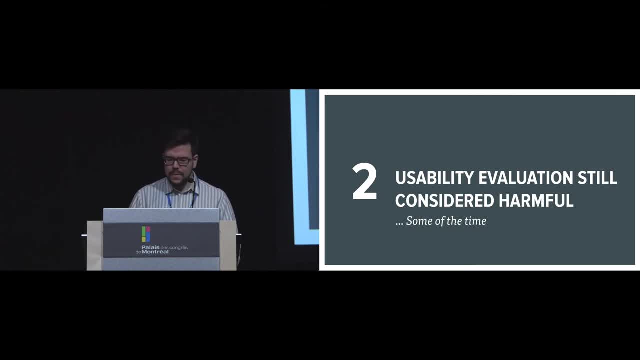 And so by doing this, the usage studies at best play a minor role in establishing and evaluating the novelty of the toolkit. But what's more interesting is that there's no indication whatsoever from the evaluation itself that a toolkit is actually successful Or whether the success of the evaluation 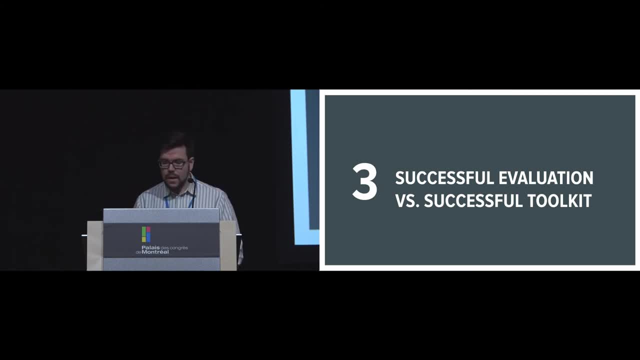 actually is tied to the success of the toolkit, because we see a lot of toolkits have enormous success within the research community, such as the Context Toolkit, And we have toolkits that are widely used outside of research as well, like d3.. 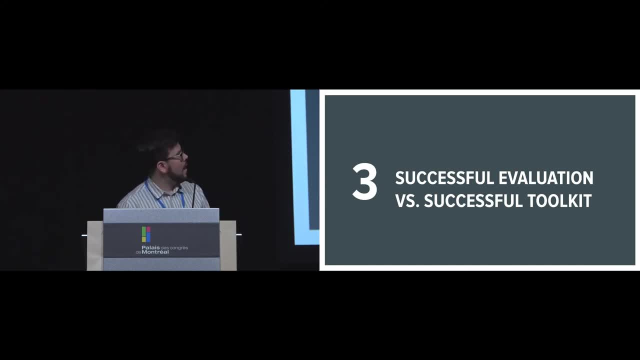 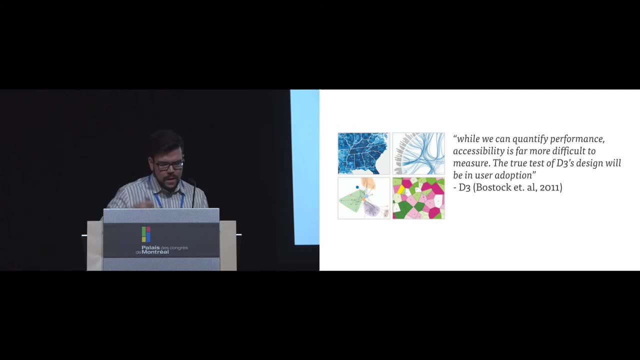 So the fact that this paper has looked at how, how they actually did that. If you read D3, they actually state this And they say that while we can quantify performance, accessibility is far more difficult to measure. The true test of D3's design will be user adoption. 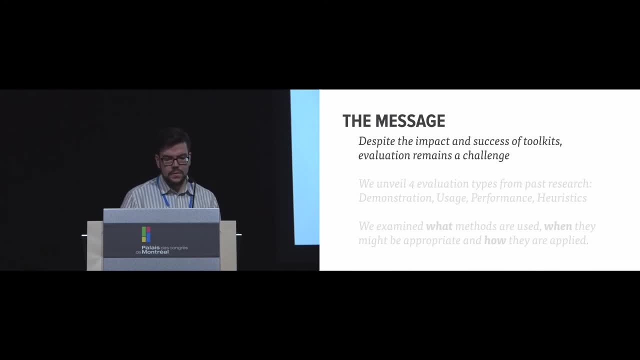 So I'll just reiterate the message one more time. Despite the impact and success of Toolkits, evaluation remains a challenge. We unveiled four different types of evaluation techniques based on past research, demonstration, usage performance and heuristics, And we examined what methods are used. 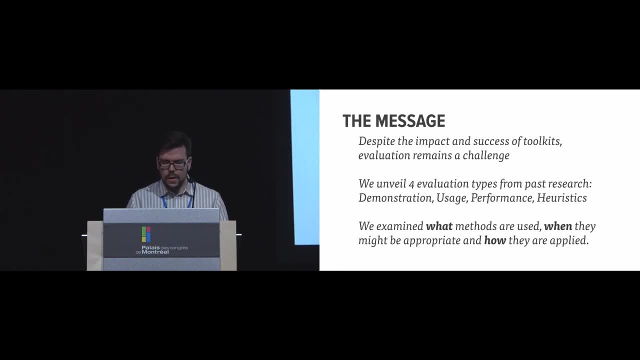 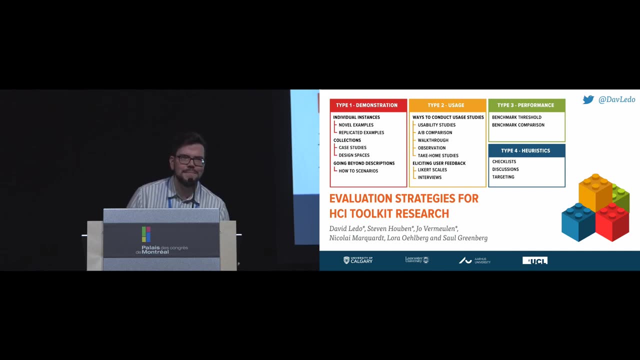 when they might be appropriate and how they're applied, And this is the first attempt in doing so And we hope that it can help HCI Toolkit research move forward. Thank you very much for your time. All right, thank you very much. 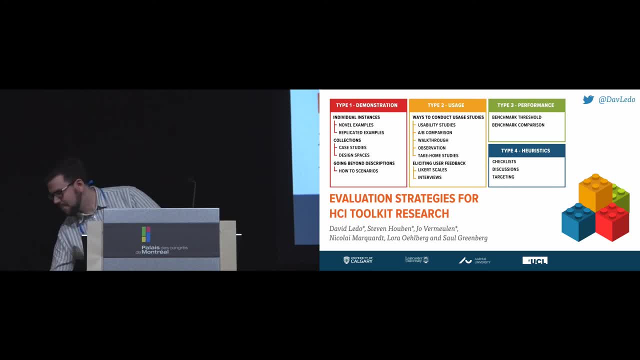 Questions from the audience, please Hi. Excellent paper. I enjoyed it very much. However, I want to ask a sort of broad question. Doesn't any kind of evaluation research method presume that you have a certain goal in mind? And one goal I would suggest is that you might evaluate? is 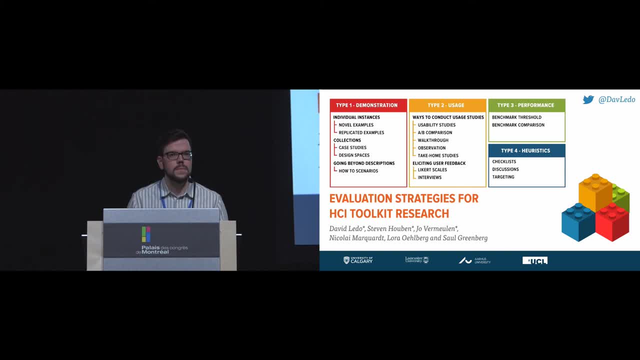 to what extent are these Toolkits being adopted by people who are producing actual products and commercial software, et cetera? Now, Now, that's not the only goal, but it would be one, And, more generally, I think, adoption against any purpose. 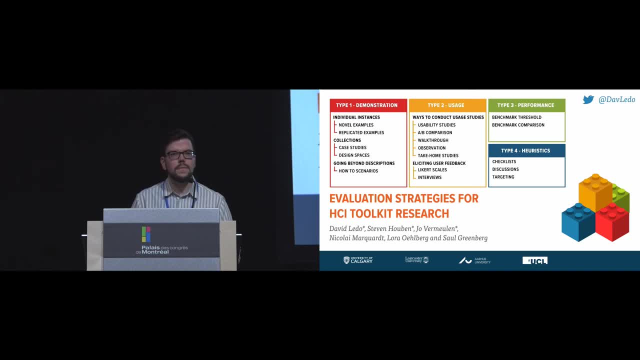 is probably the best form of evaluation. The others are more predictors of success rather than evaluation of success. Thanks for your question. Yeah, I think that's a really good point, But also we found that a lot of papers- actually because you have a Toolkit- it was able to trigger discussion. 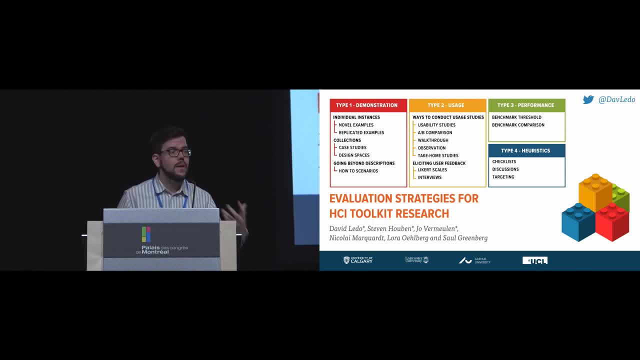 So, for example, the Context Toolkit actually created a lot of discussion behind what it means to have context awareness, And there were a lot of papers that were following up on that. So I think that it depends on what it is that the researchers are focusing on. 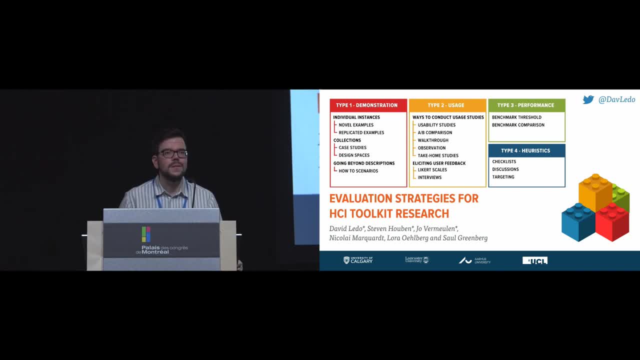 But yeah, definitely adoption is one of those really important ones, for sure. Hi, David Cargill, MIT. This is very interesting. I'm curious, though, about the sort of biased nature of the sample that you only looked at papers that were published. 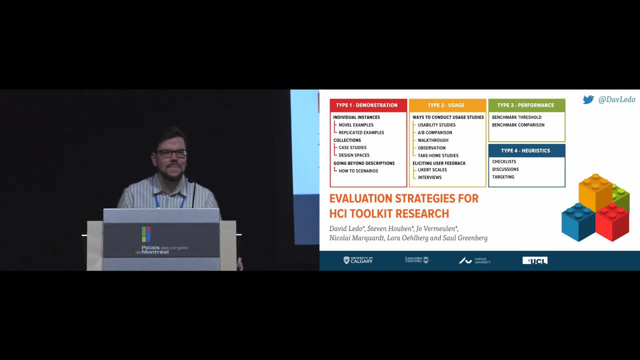 Mm-hmm, Um, And I wondered. I wonder if you have thought about whether it might be possible to get access to rejected papers and see if they have similar patterns or sort of what are failure modes and so forth. Yeah, and also not just that, but it. 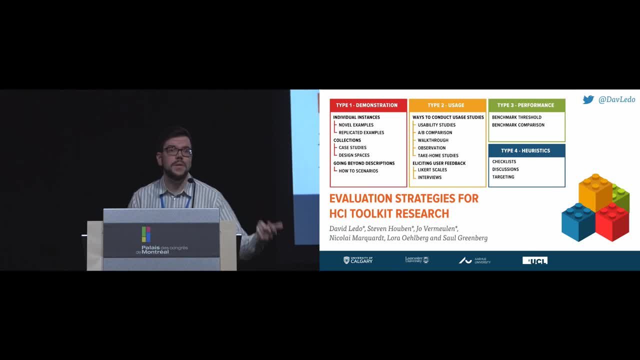 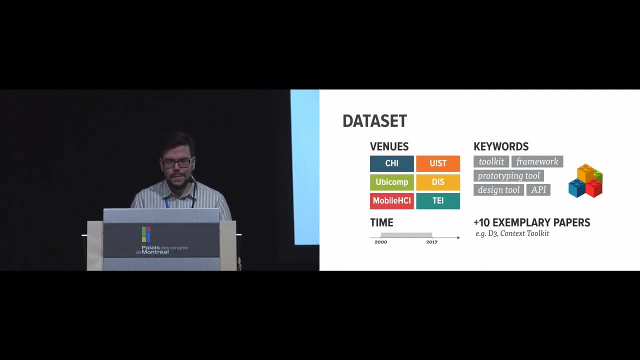 would be interesting to see if papers were rejected and because of that they had to add a user study in the end, or something like that. So in our data, yeah, it's very much biased by the things that are already out.